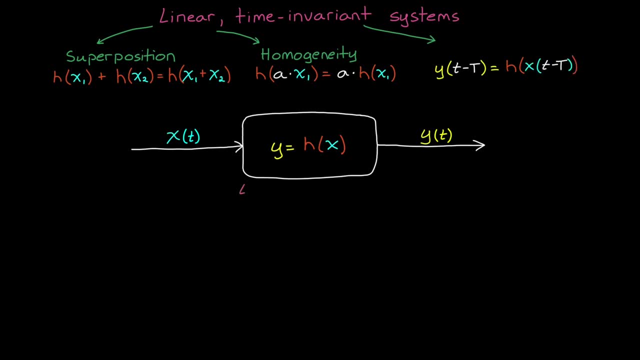 over time, And the reason LTI systems are important is because they are mathematically easy to work with and to understand. The tools that we have to analyze an LTI system are much more capable than what we have to analyze and understand non-LTI systems. 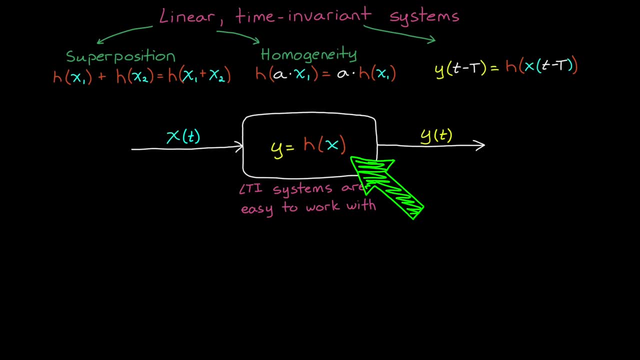 So if the thing that you're working on can be approximated and modeled as LTI, then that can make design and analysis much easier. And the main thing that we need to realize with LTI systems, for this video at least, is how the linear dynamics affect the signals that are fed into them. 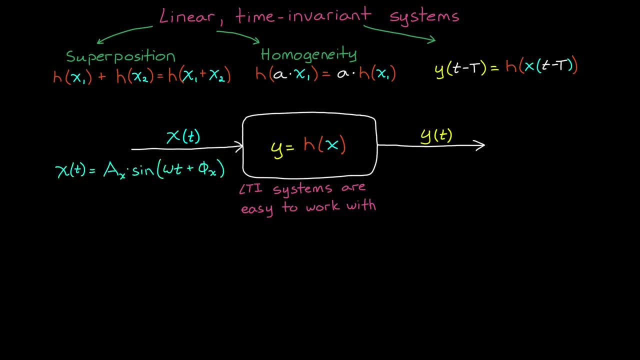 If the input is a sine wave with a frequency of omega, amplitude A and phase phi, then what comes out the other side is still a sine wave at the exact same frequency, but with a potentially different amplitude and phase. So an LTI system won't affect the 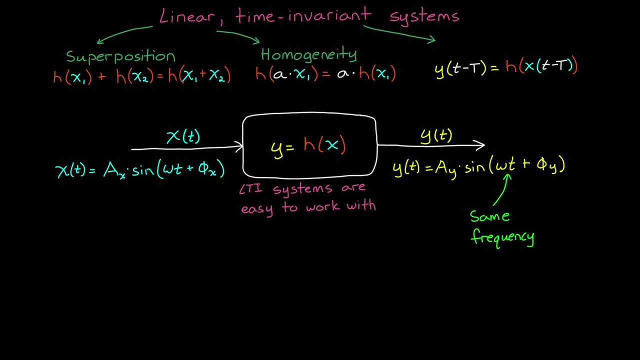 frequency or change the shape of a sinusoid, but it will affect the gain and the phase of the signal, And the amount of gain and phase depends on the frequency of the input. Therefore, we can fully describe an LTI system by looking at how it changes the gain and phase of every single frequency across the spectrum. 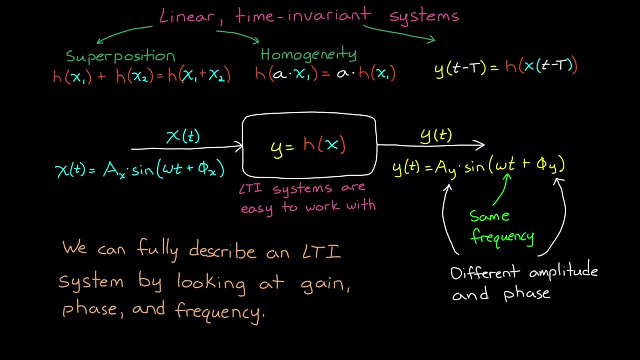 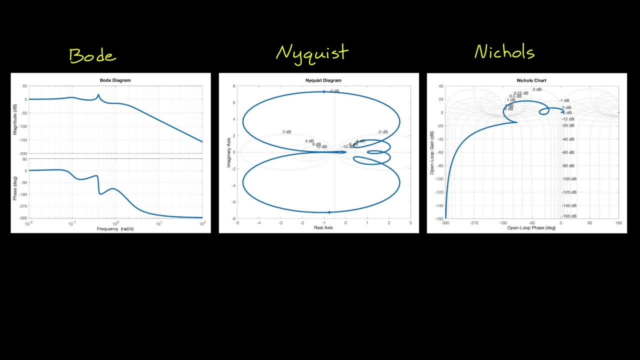 So there are three parameters that we're concerned with: gain, phase and frequency, And those are what we're looking for, And those are what we're looking for. Bode plots, Nyquist plots and Nichols plots are displaying, They all display the gain and the 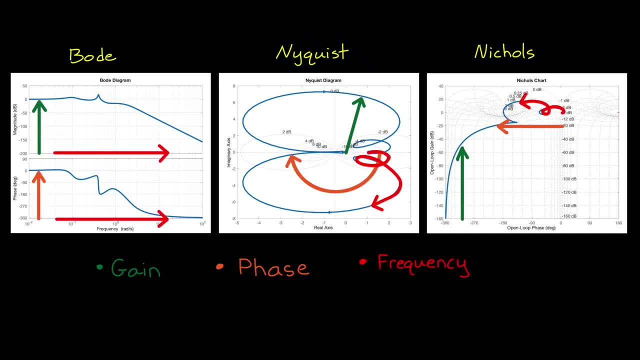 phase shift for every single frequency. It's just presented differently depending on how you want to see the data. Now, in addition to displaying these parameters neatly in graphical form, these plots are also helpful for system identification and closed loop controller design. Let's start with. 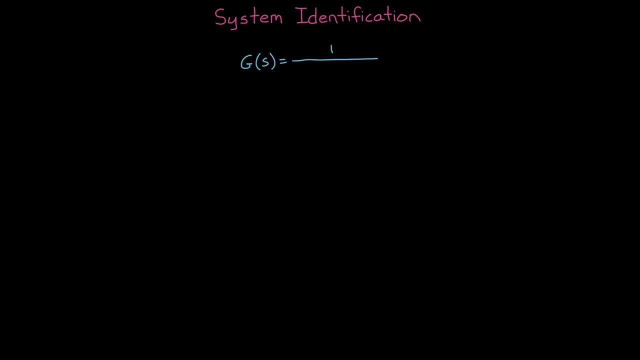 system identification. Let's say that our system can be modeled by this transfer function To generate a Bode, Nyquist or Nichols plot. we could solve the transfer function mathematically and draw the curves using the equations that we come up with. However, this method assumes that we 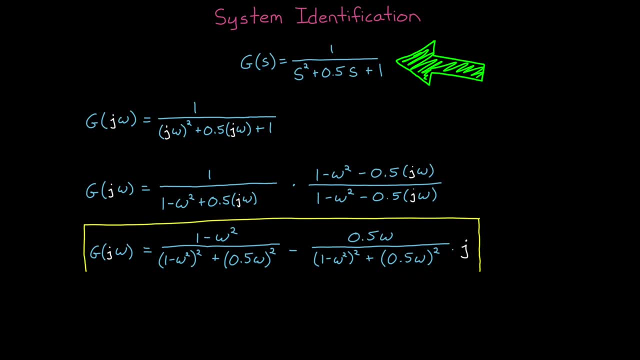 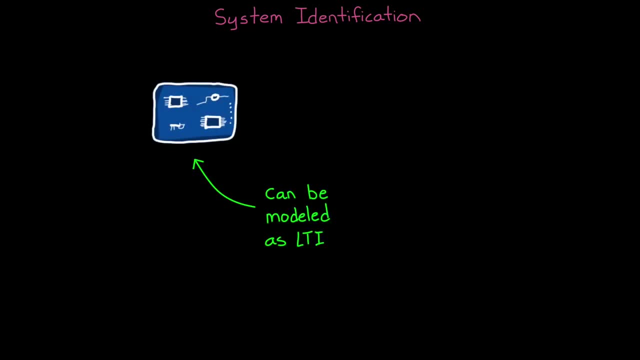 already have the transfer function to start with. So let's assume that we don't have this model. We're working with the hardware directly, like a physical electrical circuit. We know that this can be modeled as an LTI system, but we cannot really interpret it that way. Now let's discuss. 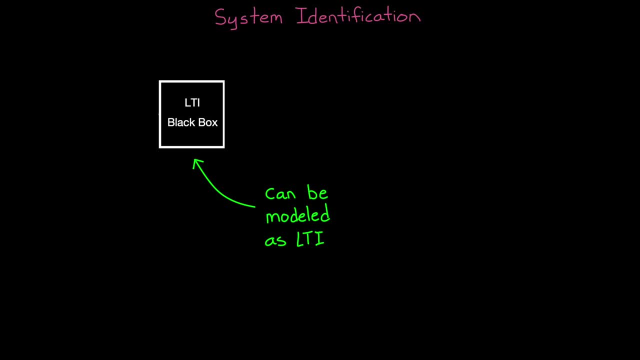 We don't yet have a model. this is just a black box to us where we can apply different inputs and measure the outputs. For instance, we could apply a voltage as a sine wave at, say, 1 radian per second and with a known amplitude, and compare it to the measured output voltage. once all of the 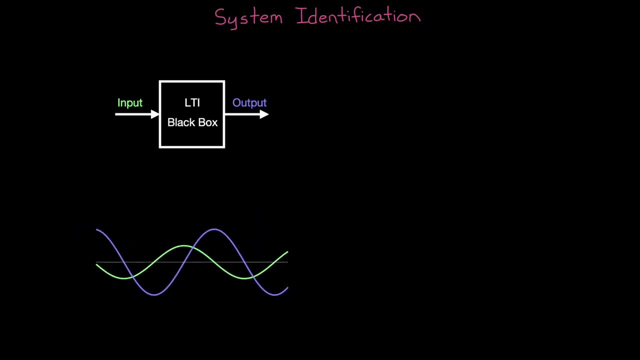 initial transients die down And by overlaying these two, we could calculate the resulting gain or change in amplitude and the resulting phase shift, In this case for a frequency of 1 radian per second. the gain increased by a factor. 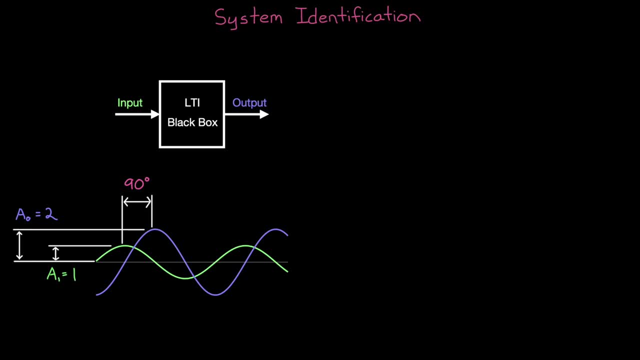 of 2, and the signal was delayed by 90 degrees of phase. Now, since gain can span such a large range, we sometimes like to represent it on a log scale. So instead of reporting a gain of 2,, we would report it in decibels, with the following: 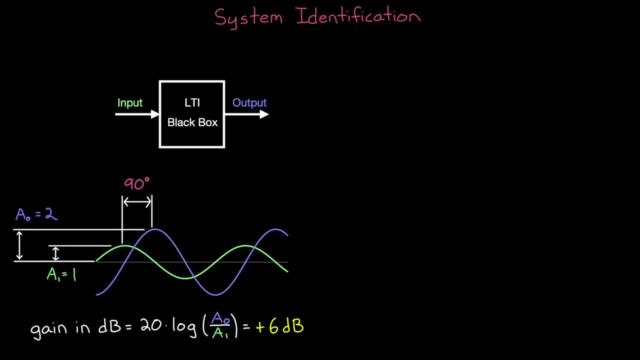 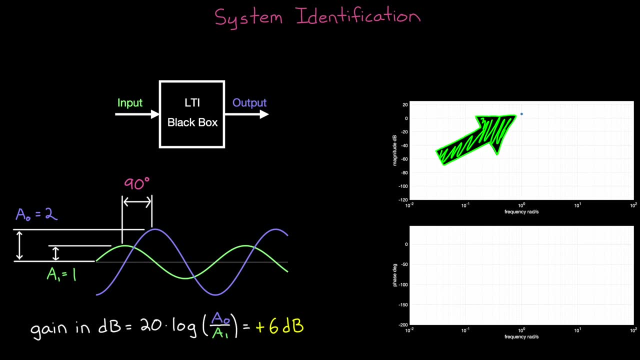 equation. So the gain here is about plus 6 dB. Alright, let's bring up two graphs. On the first we can plot this: The gain or the magnitude in dB against frequency, And on the second we can plot phase shift in degrees against frequency. 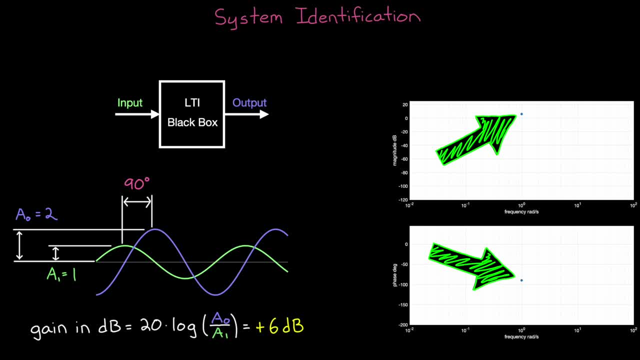 So that's our one point so far for this system, And there's not a whole lot that we can do with that, so let's get another one. I'll feed through an input voltage with a frequency of half a radian per second. 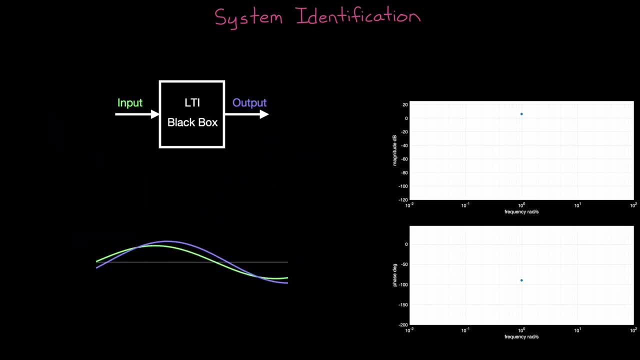 And check this out: At this slower frequency the gain is nearly 1, or 0 dB and the phase was delayed by only about 18 degrees. So overall, less of an impact, And we can add these two points on our graph. 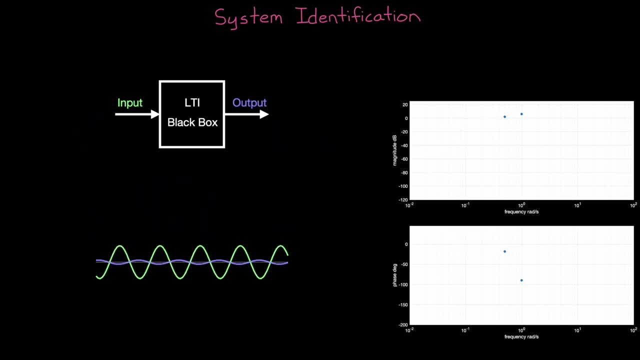 And we could choose another point at the faster 3 radians per second. And this higher frequency is attenuated by more than 18 dB And it's hard to see exactly, but the phase is delayed by about 170 degrees Now instead of one frequency at a time. if we input a signed sweep into this system, that's. 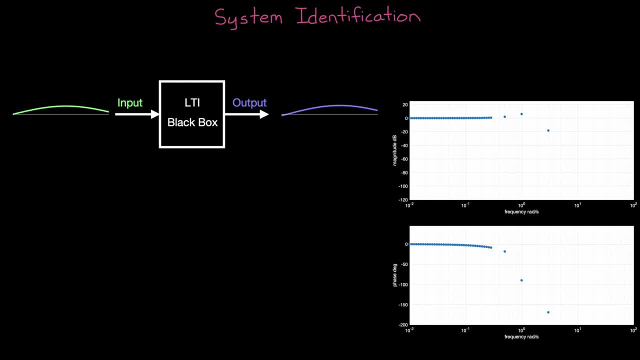 starts at some super low frequency and slowly ramps up to the high frequency inputs, we can generate the frequency response for this system And we've created a Bode plot. Remember, we don't have the model of this system. We got this information by measuring the behavior of the physical circuit. 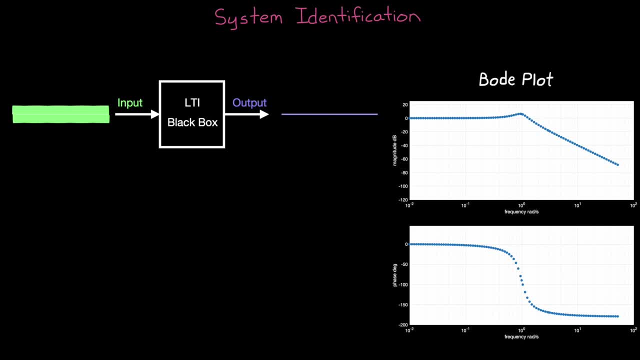 But from this information we can fit a model to this result. For example, we can see that this system has a low pass filter-like behavior, Since the low frequency signals are passed nearly unaltered and the high frequency signals are attenuated. 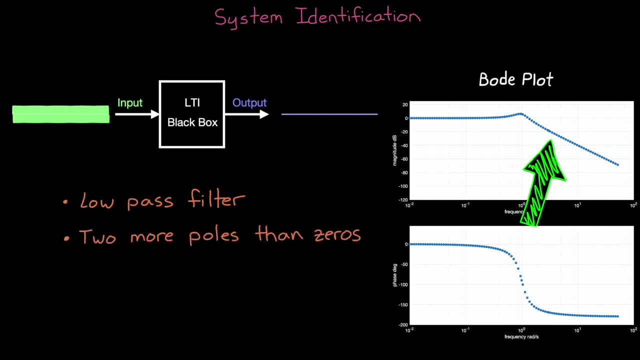 We can also tell that there are two more poles than zeros, since the magnitude at higher frequencies slope down at negative 40 dB per decade. And we can also see that there is a lightly damped mode around 1 radian per second. And by looking at this Bode plot we could fit a transfer function or a model to this. 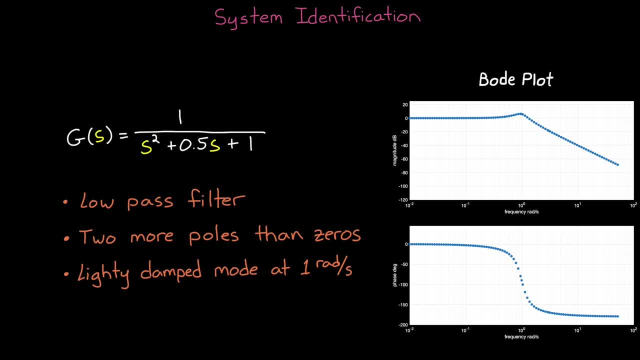 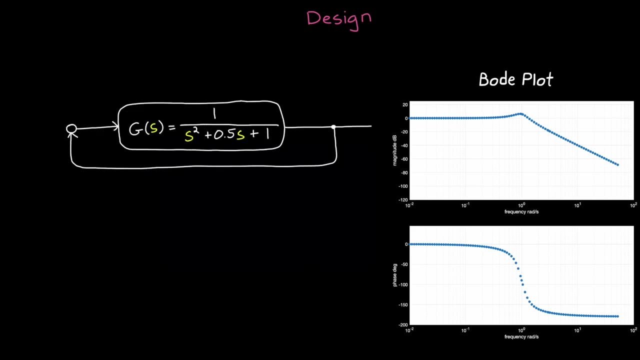 data that approximates this response. But more than just representing the system and identifying the system with data, we may also want to use this plot for design. For example, we often want to know what would happen if we wrapped a feedback controller. 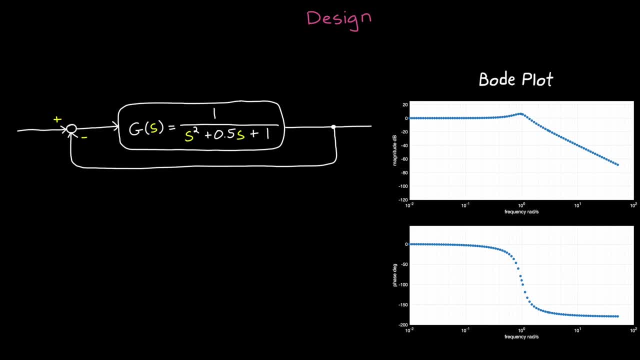 around this plant. It turns out that we can know a lot about the closed loop behavior by looking at the frequency response of the open loop system, For instance. if there are any frequencies where the open loop system is at a higher frequency than the closed loop system, we can look at the Bode plot and check if there. 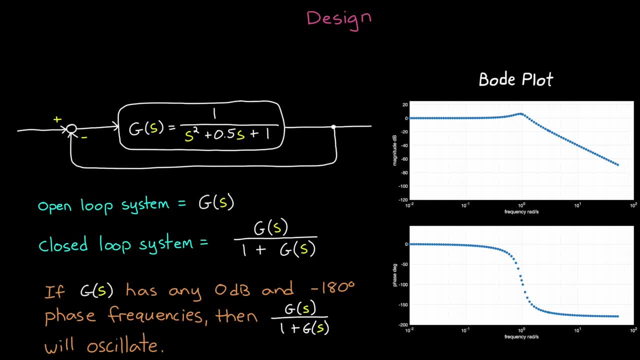 are any frequencies where the open loop system is at a lower frequency than the closed loop system. If the open loop system produces a gain of 0 dB and a phase of minus 180 degrees, this will cause an oscillation in the closed loop system. 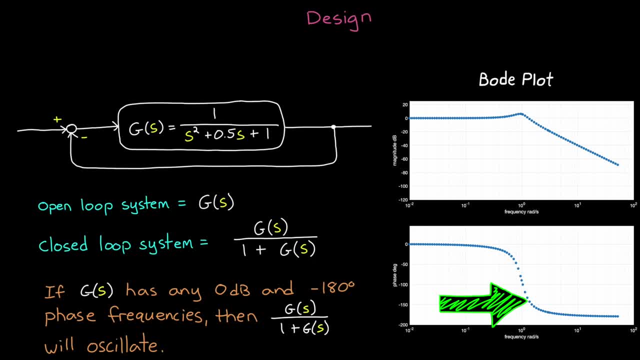 So, without actually having to close the loop and test it, we know that an open loop system with this behavior will be a bad closed loop design. So the closed loop system won't have any undamped oscillations. Of course, oscillation isn't the only thing we're concerned with. 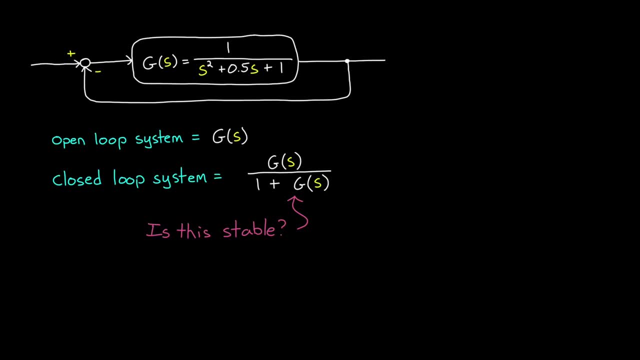 We also want to know if the closed loop system is stable. But here's where things can get a bit confusing and I apologize if my super-fast explanation adds to the confusion, But let me give it a shot anyway. If the open loop system is minimum phase and stable, so both its poles and zeros are in. 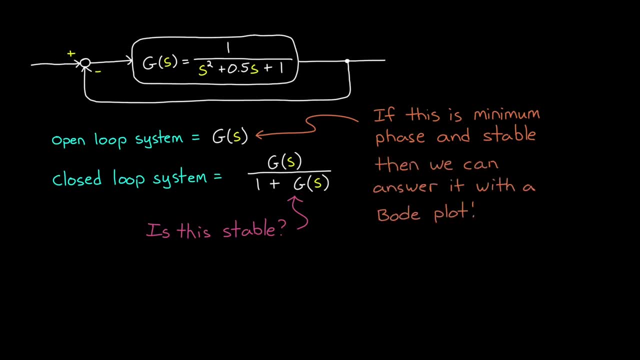 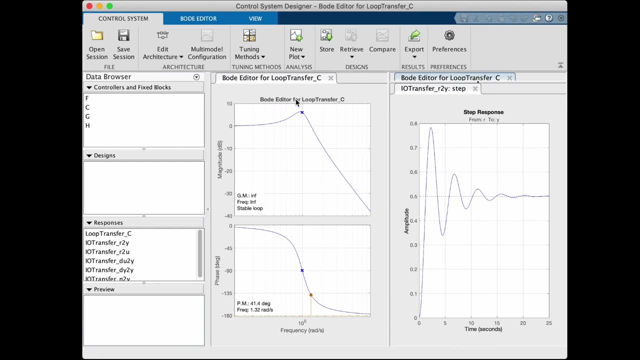 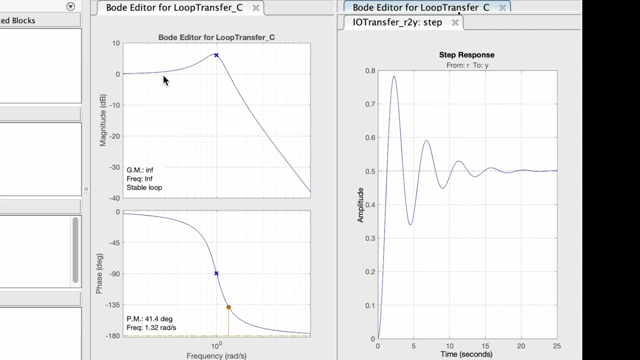 the left half plane. then we can determine closed loop stability easily from a Bode plot. This is a Bode plot for a stable minimum phase open loop system As long as the magnitude is not above 0 dB. when the phase is negative 180 degrees or 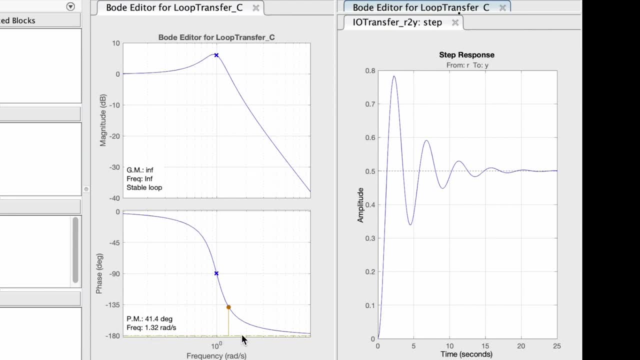 the phase is lower than negative 180 degrees. when the magnitude is 0 dB, then the closed loop system will be stable, Which is the case for this particular system, And you can see that the closed loop step response is, in fact, stable. 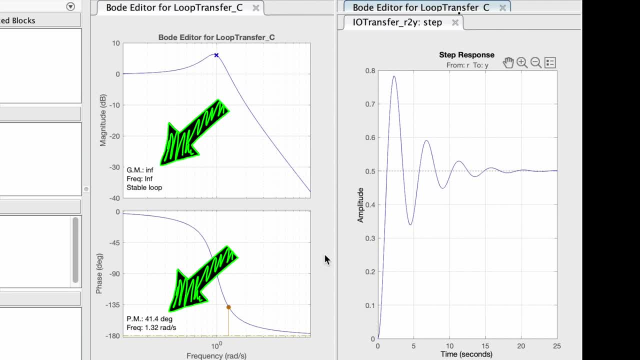 So when we're dealing with these types of open loop systems, we often see gain and phase margin displayed on a frequency response plot. This is how much the open loop system can increase in gain or phase before the closed loop system goes unstable, before the curve goes beyond the critical point. 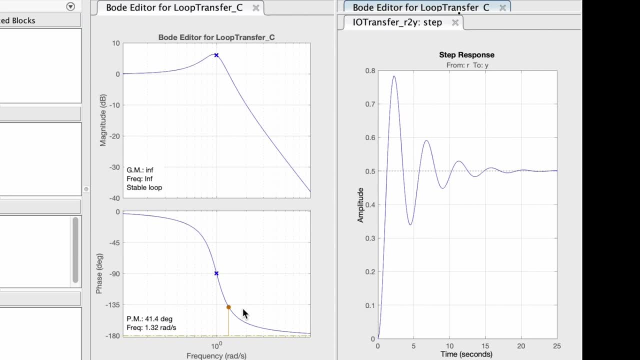 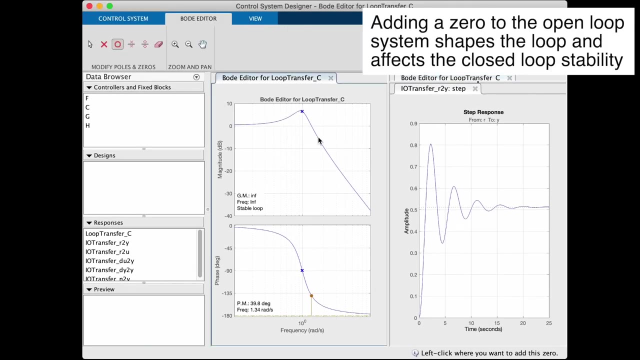 And loop shaping is the act of adding gain And poles And zeros To the open loop system in the form of a controller to get the gain and phase margin and the performance that you want for the closed loop system. And we can use a Bode plot to see where we need to shape the response to get the stability. 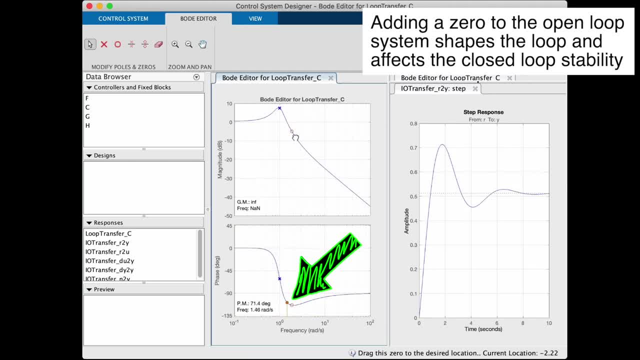 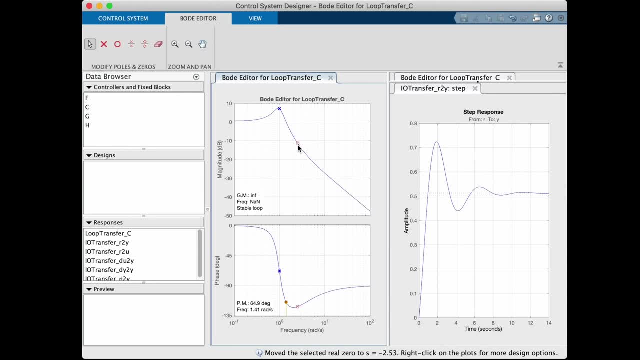 margins that we need, And we can see how close our design is to becoming unstable. Now, with all of that being said, checking for closed loop stability with a Bode plot is not as straightforward if the open loop system is non-minimum phase. 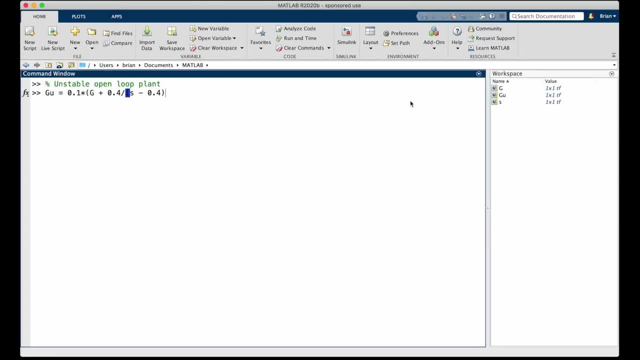 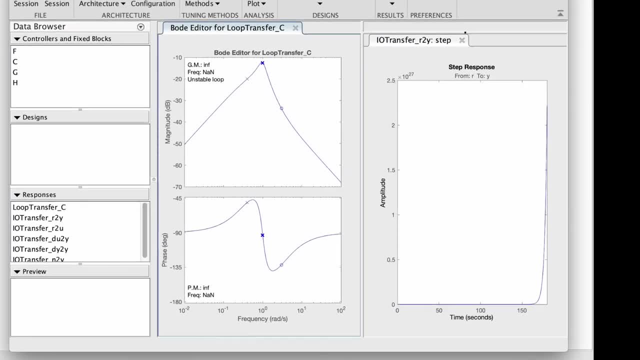 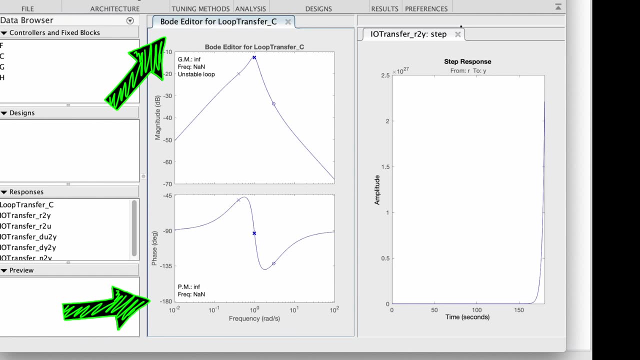 Or is unstable Here. GU is an unstable open loop system And if we check out the Bode plot for this system, it doesn't look like the response crosses either 0 dB or negative 180 degrees. So you might expect that the closed loop system will be stable. 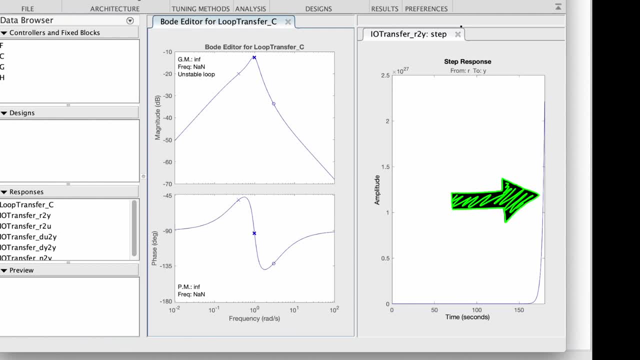 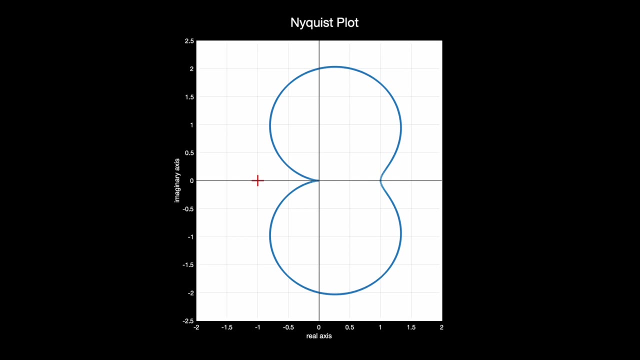 However, you can clearly see from this step response that it's unstable. So with non-minimum phase or unstable plants, a Bode plot can be unstable, And so this is where a Nyquist plot is useful. A Nyquist plot still displays gain, phase and frequency, but it does so all on a single. 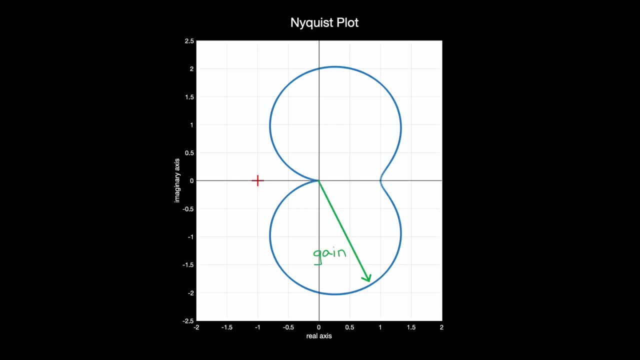 chart and with polar coordinates, Gain is the radial component, or the distance from the origin on a linear scale, so we're not dealing with decibels here- And phase is the angular component, or distance around the origin, And frequency isn't shown directly. 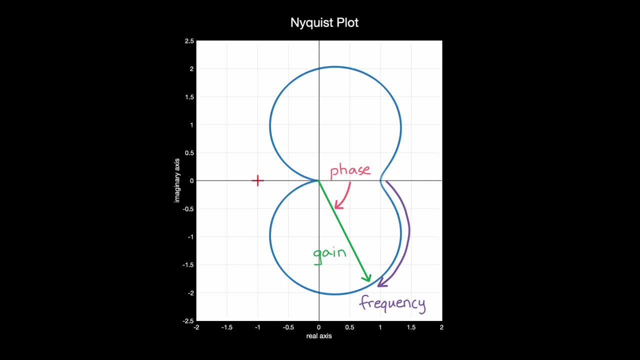 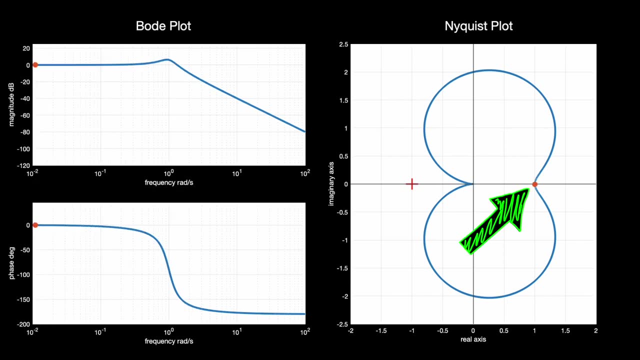 But as we progress along this curve, The frequency is changing. So if we compare this to the Bode plot, we can see that this point here has a phase shift of 0 degrees and a gain of 1. Which is 0 decibels. but again, we're not using decibels for a Nyquist plot. 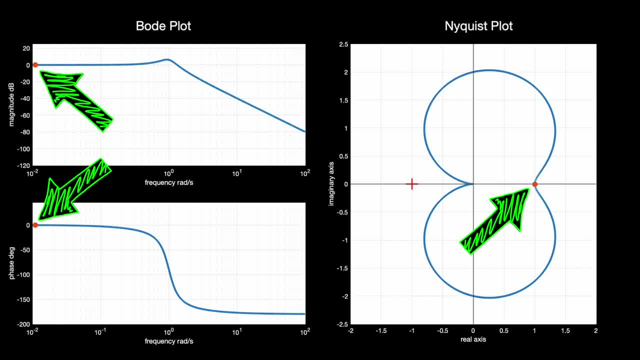 And, as we can see on the Bode plot, it corresponds to a very low frequency. And if we increase frequency until we get to 1 radian per second, we can see that this is the max gain, Or the furthest point from the origin. 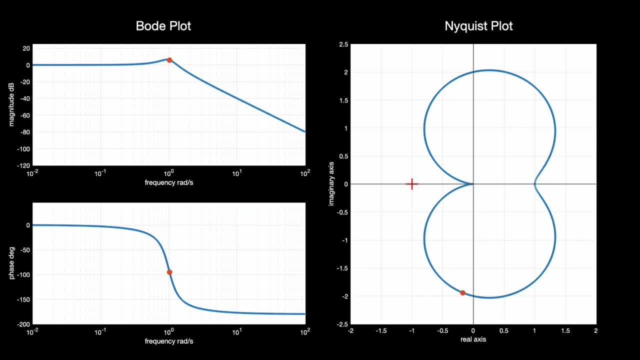 And it has a phase shift of about negative 90 degrees And at the higher frequencies, where this system has very low gain, the Nyquist plot tends towards the origin. Now the upper half of the Nyquist plot is a mirror image of the lower half. 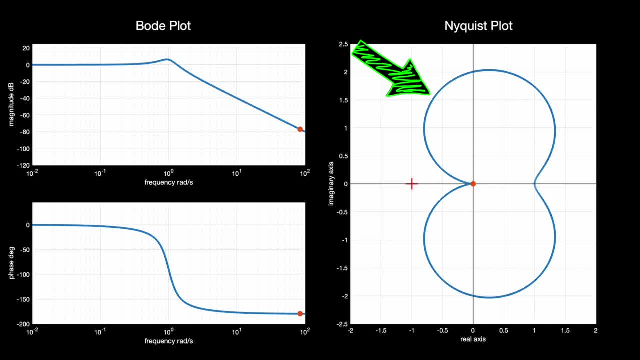 And it shows the response for negative frequencies Which are typically not shown on the Bode plot. Also, notice the critical point, The one we're trying to avoid, for oscillations. It's just a single point on a Nyquist plot And it corresponds to negative 180 degrees and a gain of 1.. 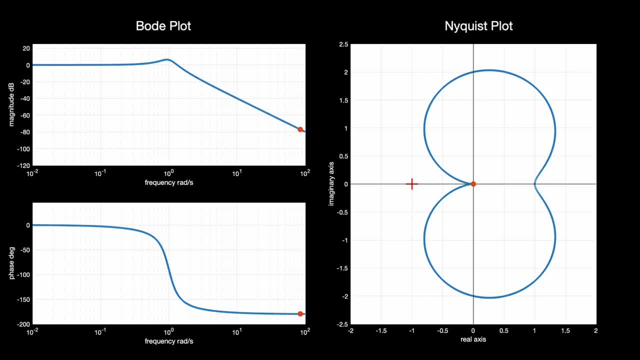 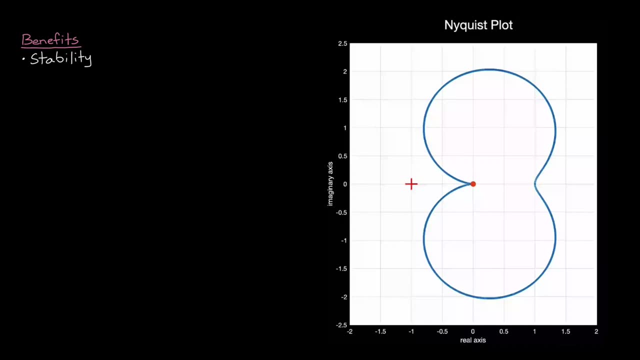 So this is how the Nyquist plot packages the exact same data that we have in the Bode plot. But the question now might be: why are we even displaying the data in this form? And there are some pretty good reasons. One is that we can determine closed loop stability much easier with this format. 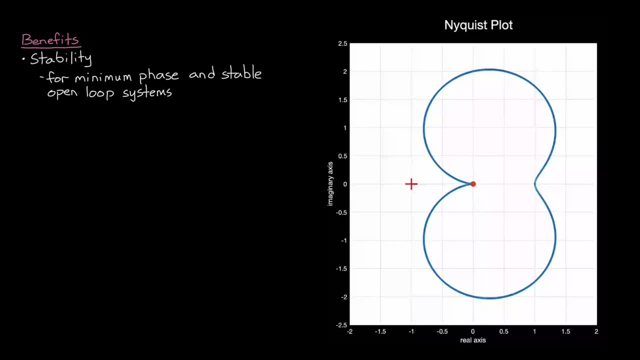 If the open loop system is minimum phase and stable, Then, just like with the Bode plot, we can claim that the closed loop system is stable, as long as the curve doesn't cross over this critical point And since all of the information is presented in a single graph and there's only a single, 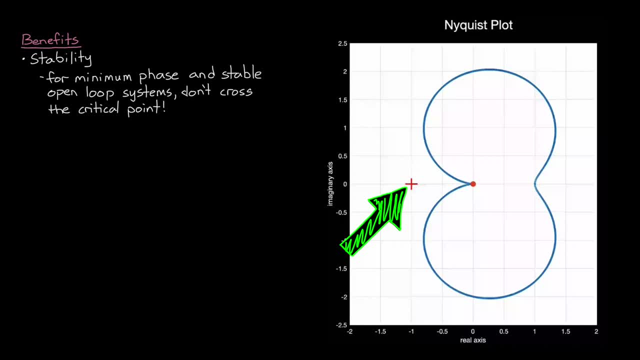 critical point. we can see very clearly how close the curve is to it, Even if there are multiple close passes, And gain and phase margin can still be read directly off this chart, just like we can with a Bode plot. Also, The benefit of a single plot like this is that we can more easily see how combinations 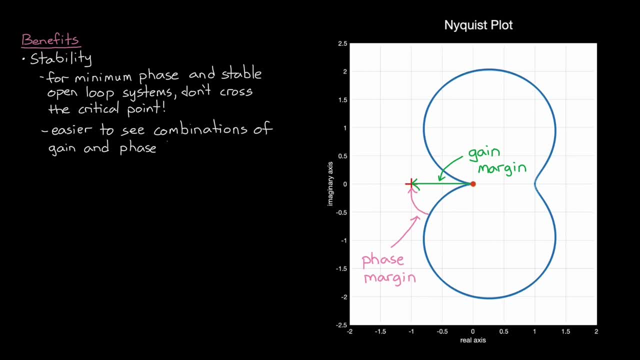 of gain and phase impact the stability of the system. In fact, disk margin, which is arguably a better way to think about margin in your system, is built on this kind of representation. Furthermore, per the Nyquist stability criterion, we can also determine closed loop stability. 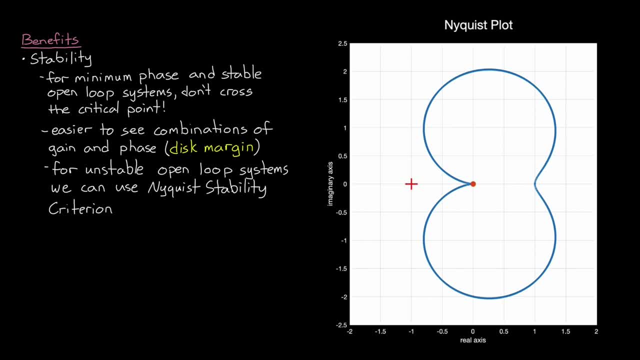 for unstable open loop systems, which is something that was very difficult to do. on a Bode plot, We can compare the number and direction of encirclements over the increase in distance, And we can also determine the number of encirclements over the increase in distance. 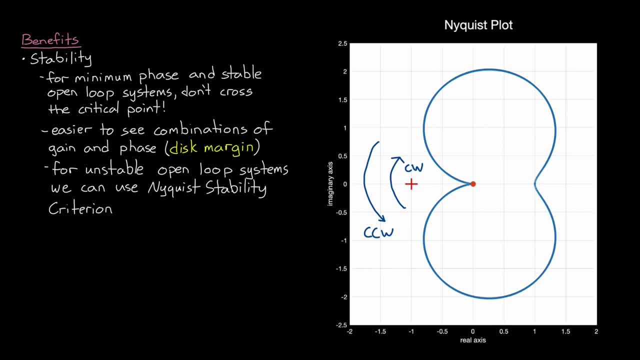 We can compare the number and direction of encirclements over the increase in distance around the critical point with the number of right half plane poles for the open loop system and then determine closed loop stability. So for certain systems it's easier to check for stability and to design a closed loop. 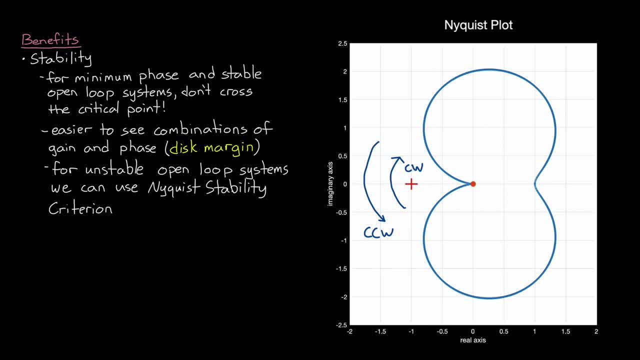 controller with a Nyquist plot than it is with a Bode plot. But the downside of Nyquist is that it tends to be harder to read, since frequency is not explicitly called out, and I find that it's not terribly intuitive to look at a Nyquist. 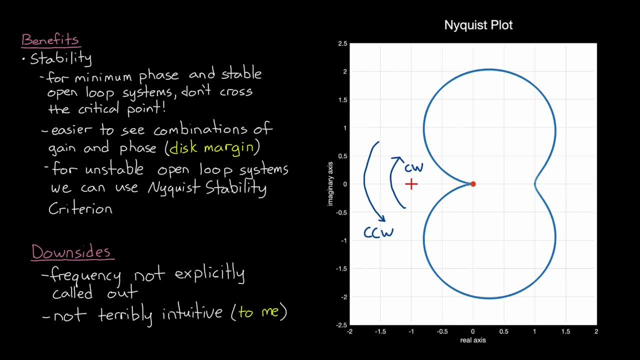 plot without a lot of practice. Of course, that's entirely a preference thing and not a statement of fact, but one of the reasons that I think it's hard to read is that it's harder to visualize an angular distance than it is a straight line distance. 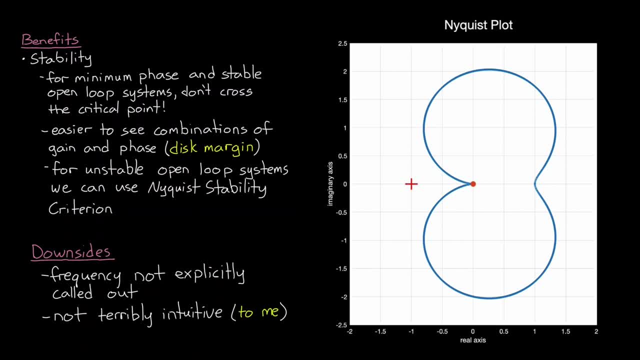 For example, how much phase margin is there in this design? Well, it's the angle between the critical point and where the curve crosses the unit circle. So, whatever this is Maybe around 45 degrees or so. Well, to find out exactly, let's go over to Matlab. 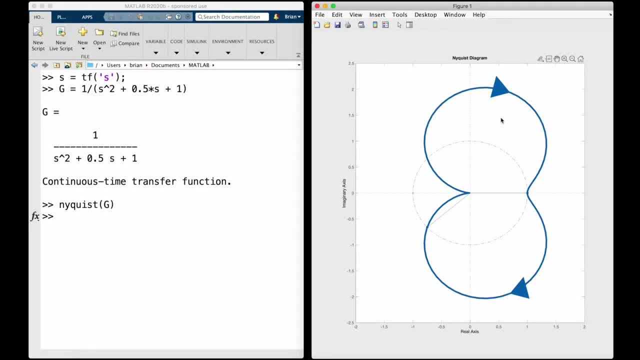 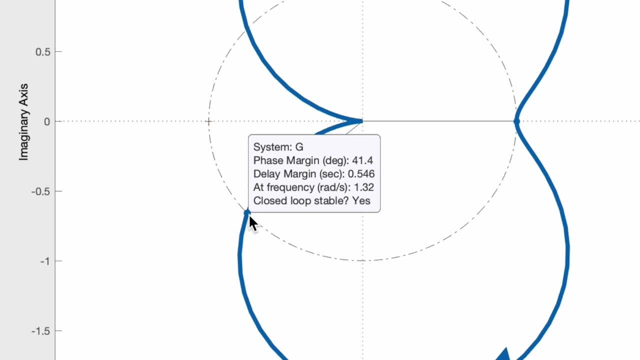 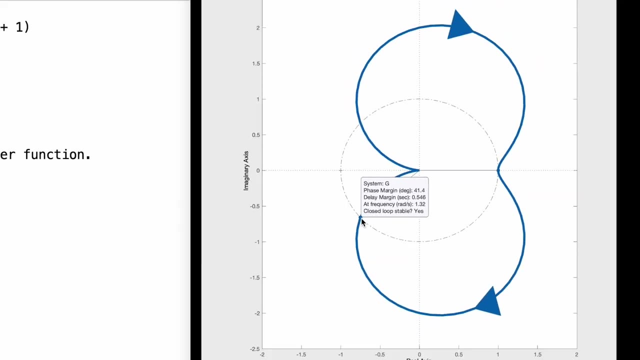 And it turns out it's about 41.4 degrees. So you can definitely read phase from this plot for sure. But my personal preference is to be able to view these margins on a Cartesian graph rather than a polar graph. Plus, on a polar graph we can create some pretty gnarly results as the response curve loops. 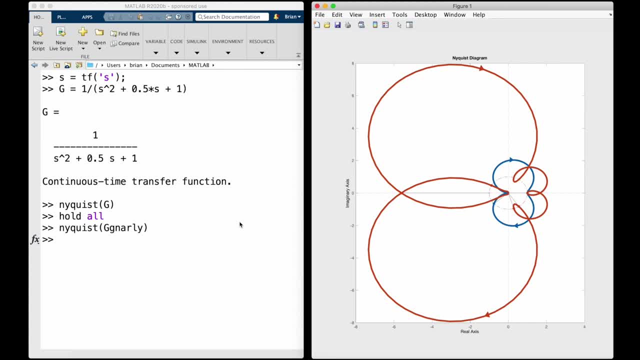 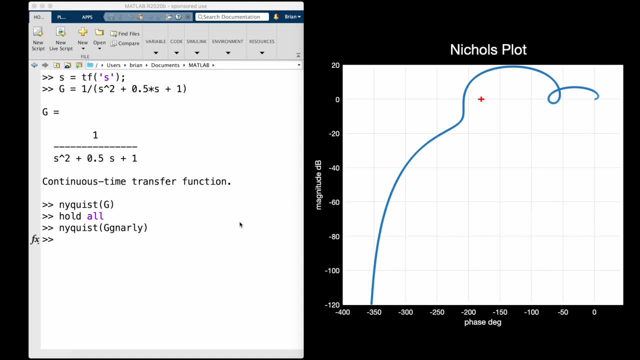 around four systems with a lot going on. So to solve this, enter the Nichols plot. Nichols is a single graph, like Nyquist, but it plots the information on a Cartesian grid. Magnitude is the vertical axis in dB and phase is the horizontal axis in degrees. 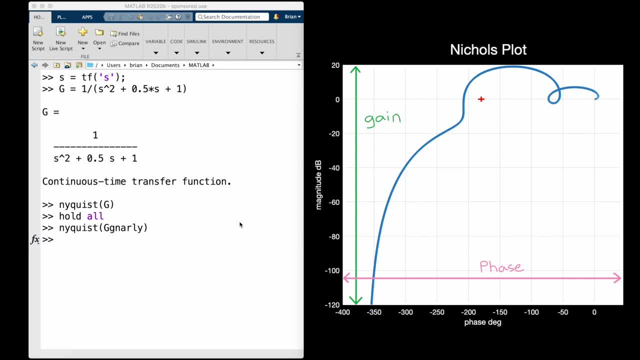 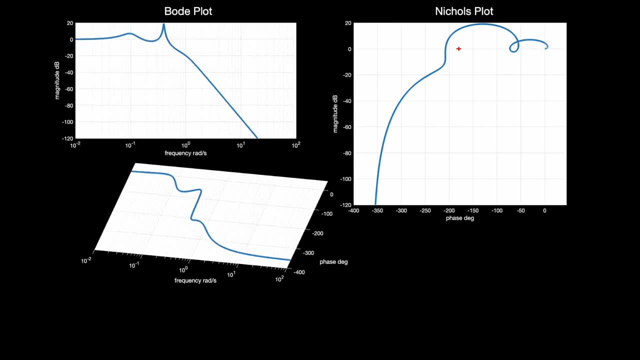 So it's the exact same units as the Bode plot. In fact it is the Bode plot information just packaged onto a single chart, And I think it's easier to visualize if we align the magnitude and phase plots with the Nichols chart. 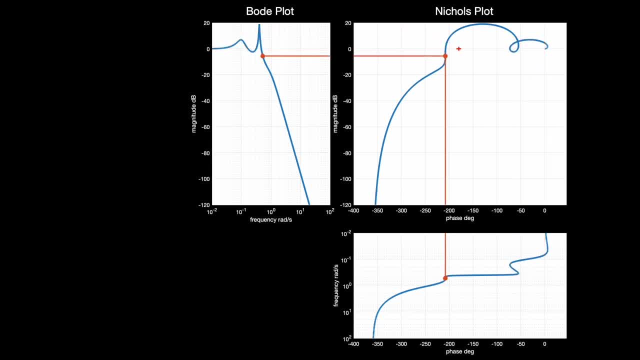 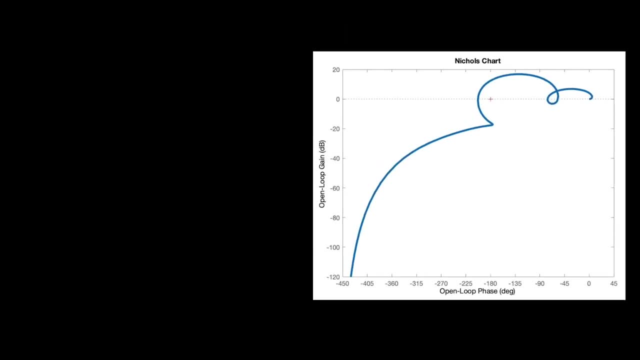 So if you look through the frequencies, you can see how the Bode plot information is mapped into this single graph. A Nichols plot has some of the same benefits as the Nyquist plot in that the information is on a single chart so that we can visually see how combinations of gain and phase will. 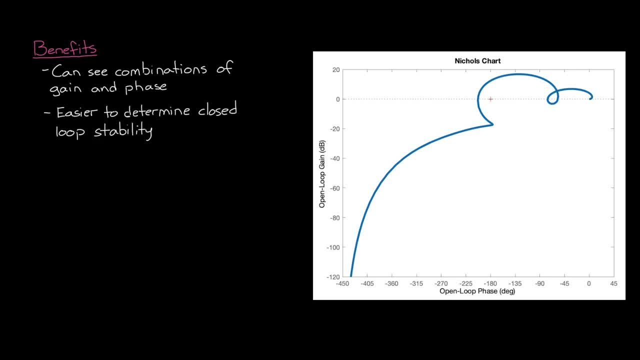 impact stability Plus, it's easier to determine stability of non-minimum phase and unstable open loop plants than it is for a Bode plot. We can apply the Nichols stability criterion to this chart as well, by counting how many times the curve crosses above the critical frequency and in which direction. 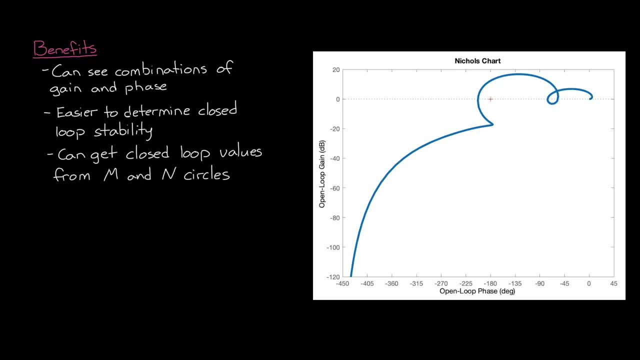 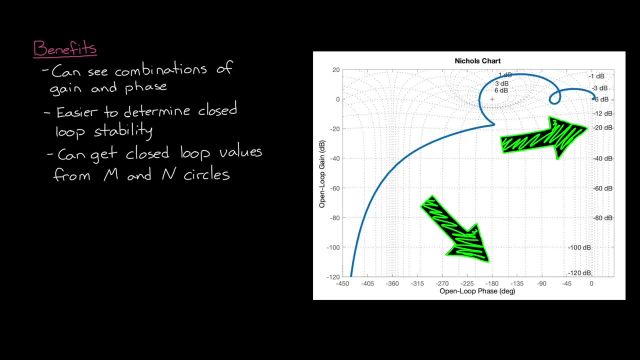 Also, when we're talking about closed loop design, we can obtain the values of the closed loop transfer function from the open loop frequency response by overlaying a grid that shows the so-called M and N circles. From this grid we can read the gain and phase of the closed loop system directly. 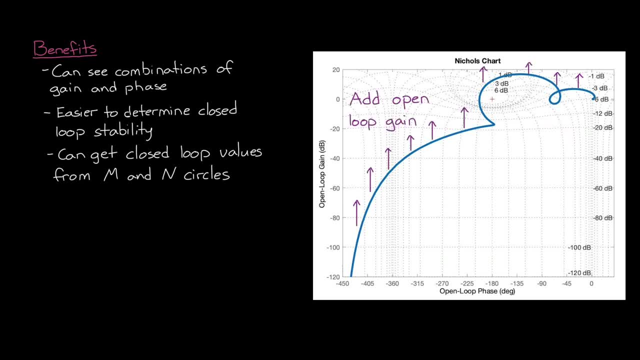 And since adjusting the open loop gain, we're able to read the gain and phase of the closed loop system directly causes the Nichols plot to move up or down with the grid. it's really easy to see how open-loop gain will affect closed-loop response. 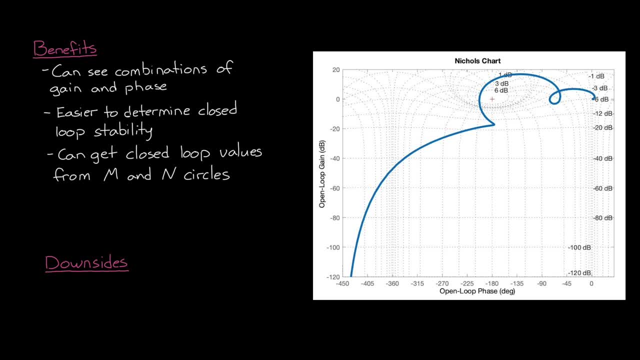 But a Nichols plot also has some of the same downsides as the Nyquist plot, in that frequency is still not explicitly called out. So Nichols and Nyquist seem pretty similar. However, the difference is that I think it can be easier to read off gain and phase on. 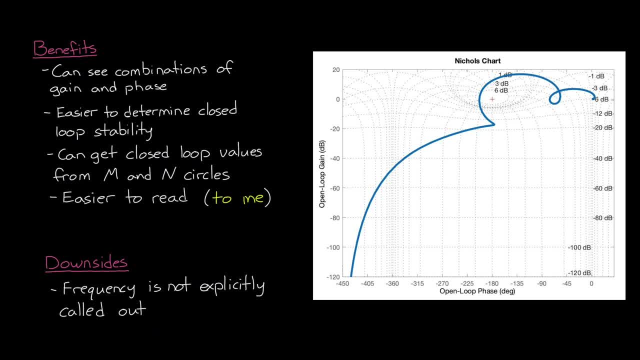 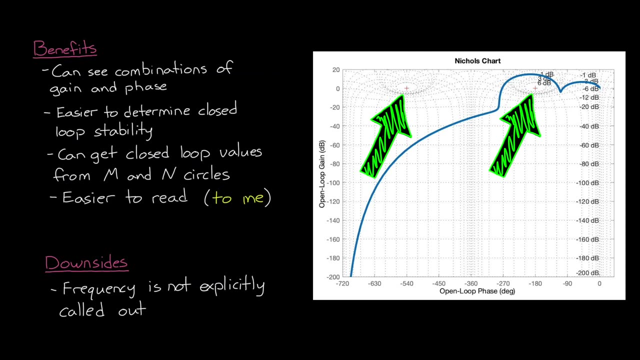 a Cartesian grid rather than a polar grid, And for open-loop systems that have a lot of phase lag rather than looping around the origin. a whole bunch like the Nyquist plot. the Nichols plot just keeps moving to the left indefinitely, adding additional critical points every 360 degrees. 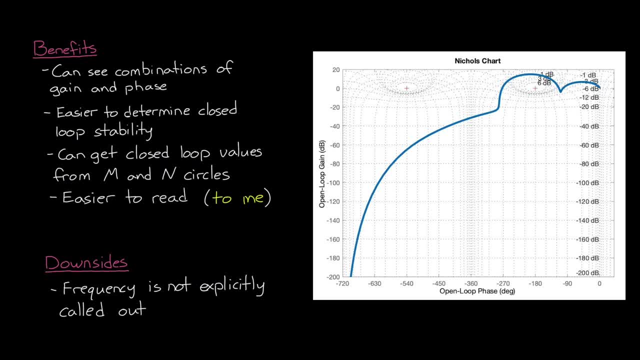 So is the Nichols plot the best? Yes, Yes, it is. Well, maybe not for everyone. The plot that you rely on the most Is more than likely the one that you're most familiar with. Like I said, they all show the same information.